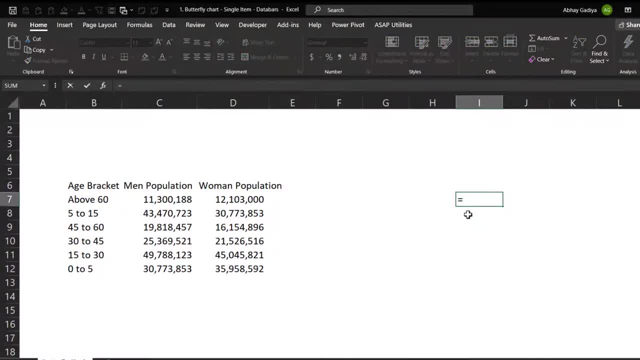 So now let me just quickly press equal to and then select this age bucket. So I will just copy this across the rows so that it gets displayed the same way. So on the left side, we want to keep women as a population, So let me copy this: 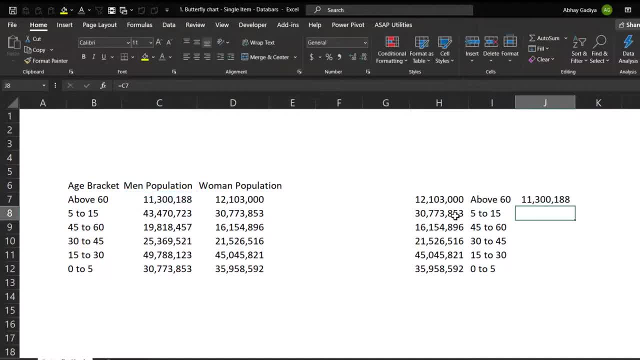 Then I will be selecting men here and let me copy this as well. So now here we can see that we have women related population and this will be men related And this is our age brackets. So let me just quickly format this, Let me decrease the font size. 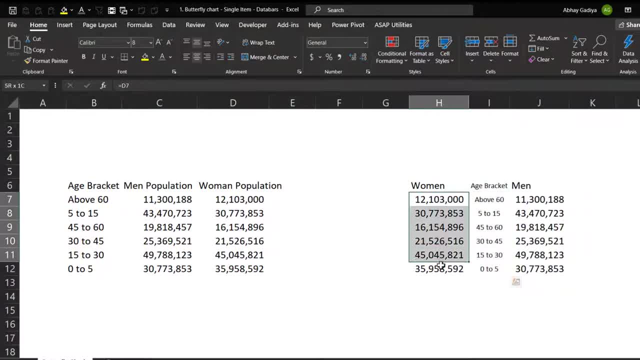 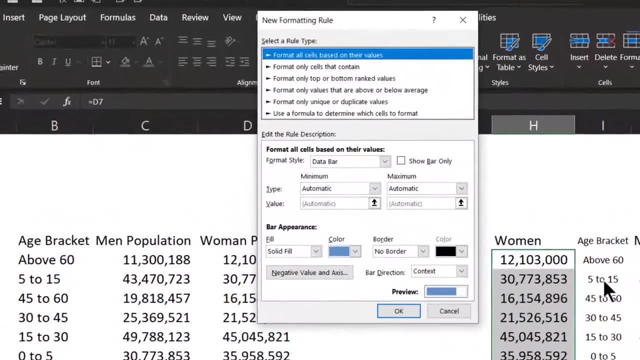 So this is fine. So now we will be quickly creating this visuals using data bars from conditional formatting. So I have selected women, Then I will have to go to data bars, select data bars and then I can click on more rules. Now I want to show only the data bars. 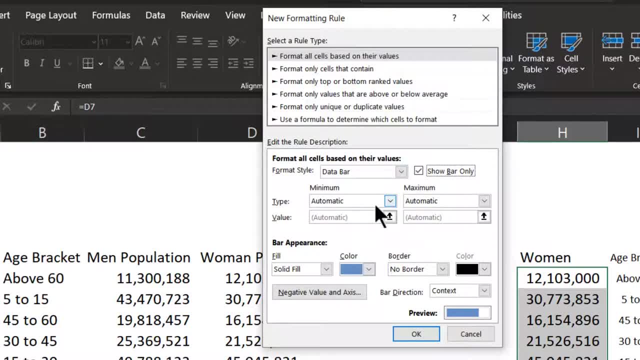 And not the numbers. So I will simply select show bar only, Then minimum value. I will keep it zero and maximum value: I will have to put it over here, or I can also select a particular cell. So for the time being I will be typing this: 55 million here. 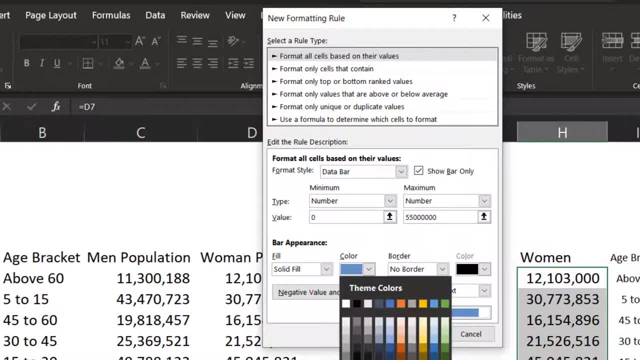 So 55 million. I have added So I can change the color. Let us say pink, and then the bar direction will be right to left. So immediately you can see our bar starts from here. So we can see that our bar chart starts from the right instead of left. 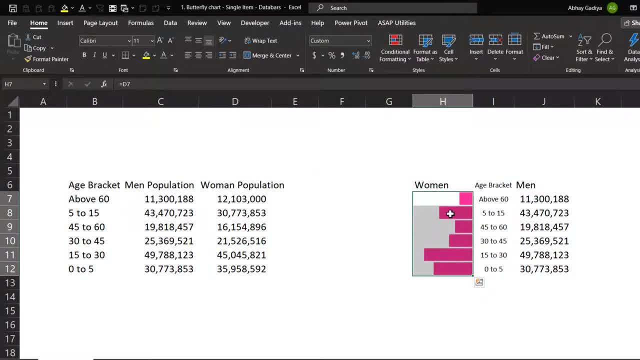 So let us click OK And here you can see our bar chart is being displayed. Same way we will do it for men, But for the time being I will be now putting some value here, which we have done for maximum value, which is 55 million. 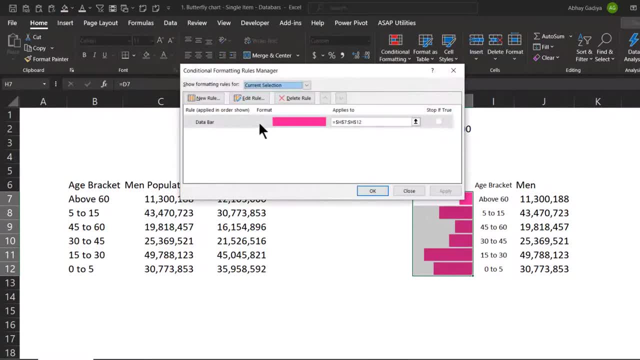 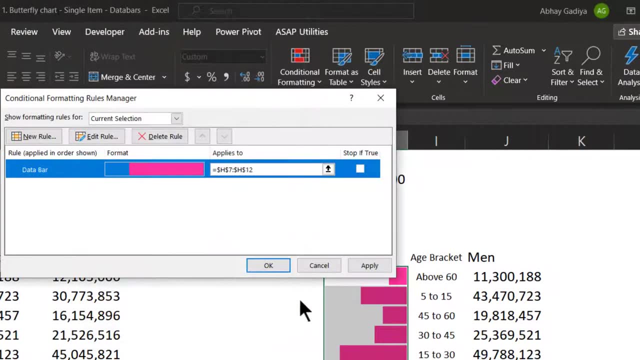 So now let me quickly refer that I can go to manage rules, select this and then click edit, And now I can select this value And let us click OK, Let us quickly say apply, so that this highest value will be common across men and women. 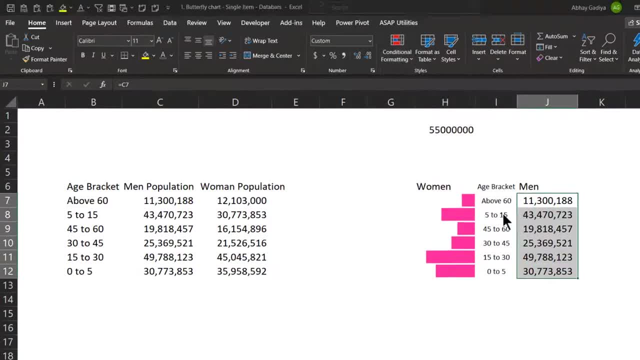 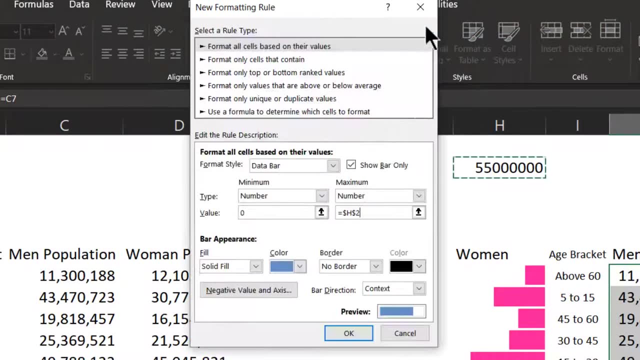 So let me now select this data. Go to data bar. more rules show bar. number. minimum will be zero maximum. I can select now this H2 as a cell, Then this color. I can change it and context left to right is fine with me. 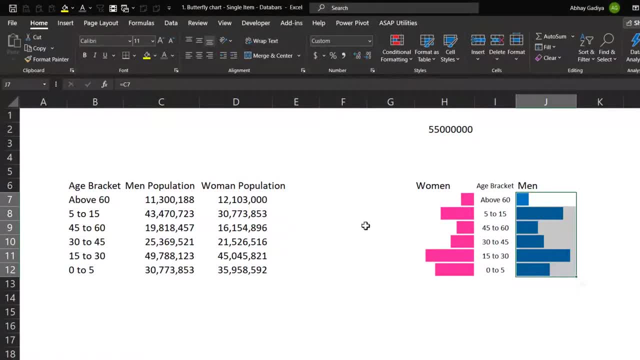 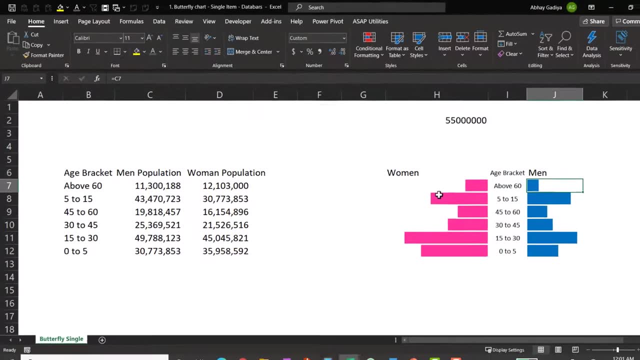 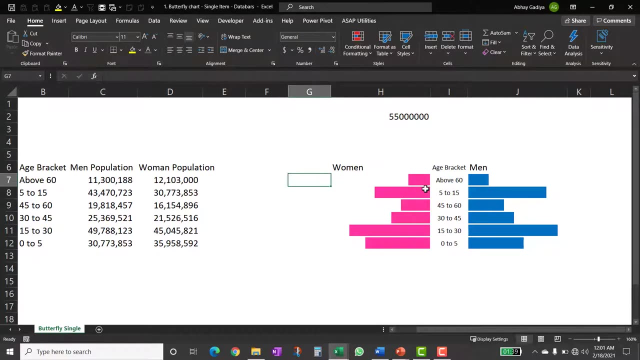 Let us click OK. So here, quickly, you can see this bar Are getting displayed, So let me quickly resize the column width for both of them so that it looks consistent. Now, column just after this: I will be just putting it as a four column width. 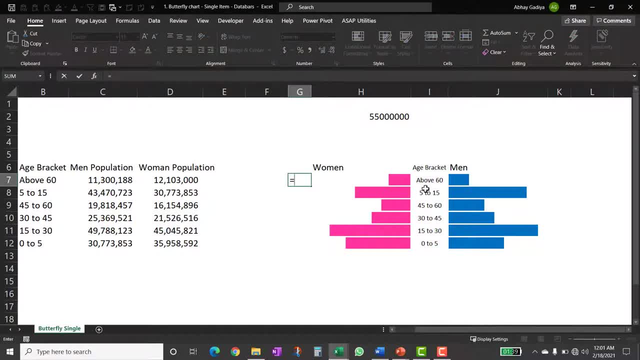 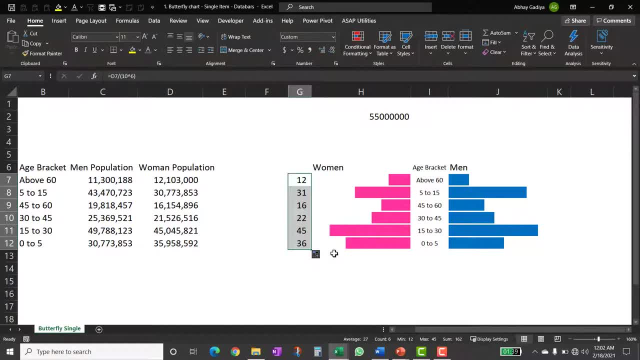 And I've got it, So that way I can just just just do it for maximum or maximum or for maximum, And we will just copy these values over here. So this will be our data levels, which we want to put it over here, And so let me quickly format this. numbers not required. 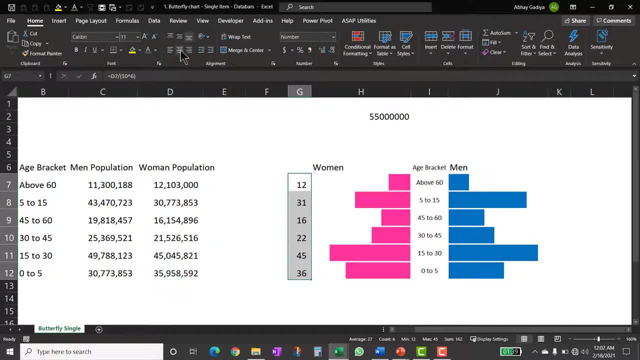 So let me just see. if he says the height of rows also to make it twenty, The list, all of them, that looks proper, This number I can put. So let me quickly select this: data divided by 10: raise to 6. bracket. close control enter. 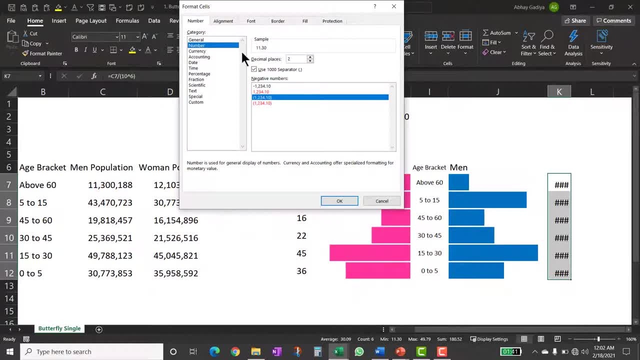 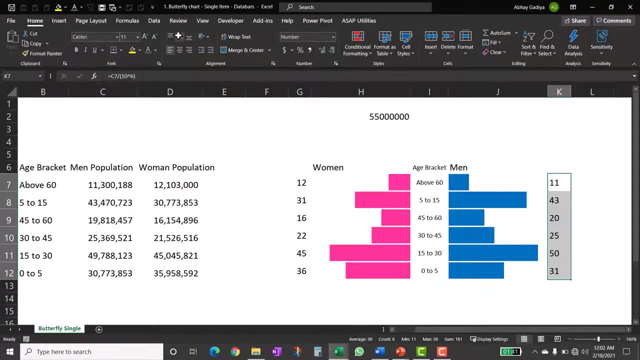 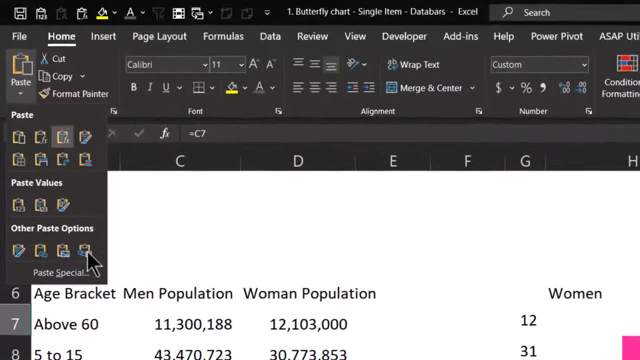 Let us quickly format this also as a number- no decimal places- and let us click ok. Let us quickly format this also in alignment. Now let us copy this and then select this cell, go to paste and then click on the last option, which is called as linked picture. 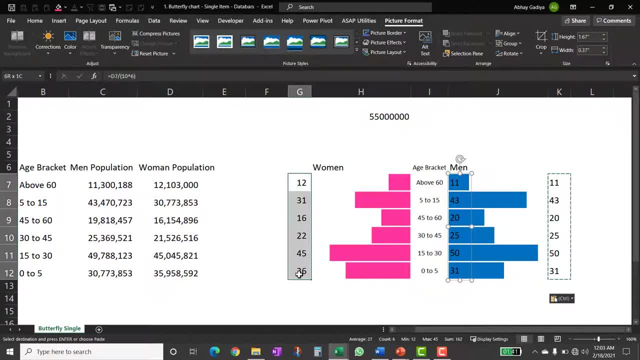 So here you can see these numbers are getting displayed. Same way, I will do it for this copy. Then select over here, go to paste and link picture. So now I can move this link picture to properly align it over here. So this looks proper to me. 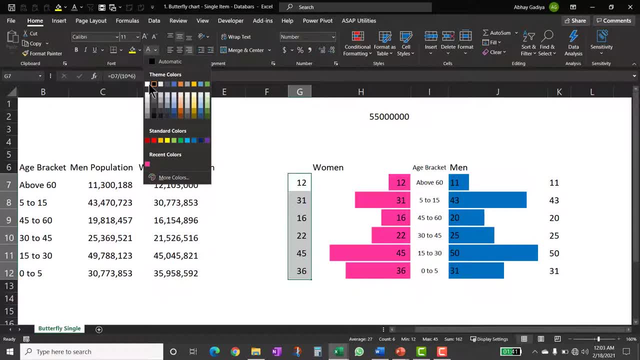 Now I can change the font color. instead of black, I can select them and click white so that it gets hidden. However, Since this text is above the colored bars, it is showing properly Same way. I will do it over here and this looks proper to me. 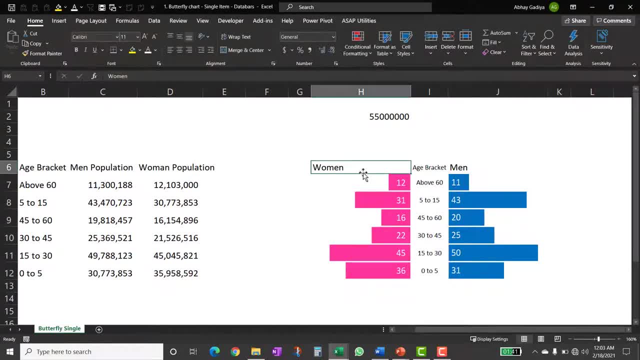 I can align it the way I want it, So women can be right aligned. men is already disaligned, So let us quickly change the color, make it bold for women also. Let us change the color and make it bold. Now, at the top, we can give the chart title. 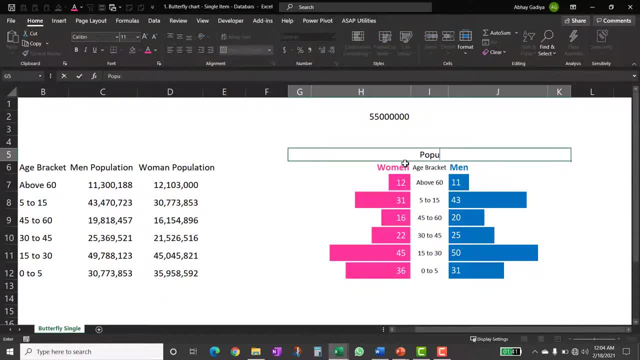 Let me, Let me first merge this population distribution numbers in millions. This is in millions, and now let me quickly decrease the font size for this, so I can make it eight. So this is fine. So let us change the font color So this one can be a bold population distribution. 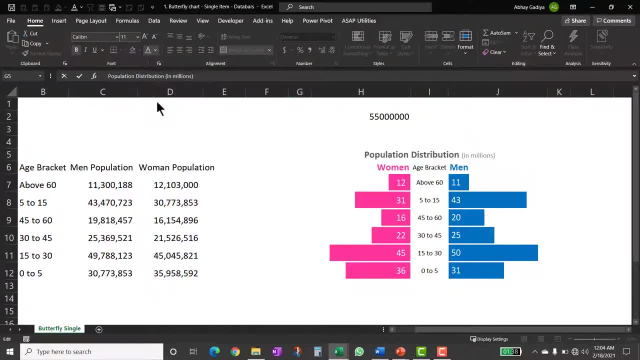 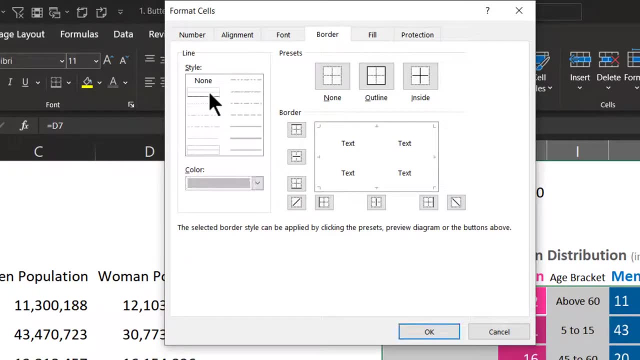 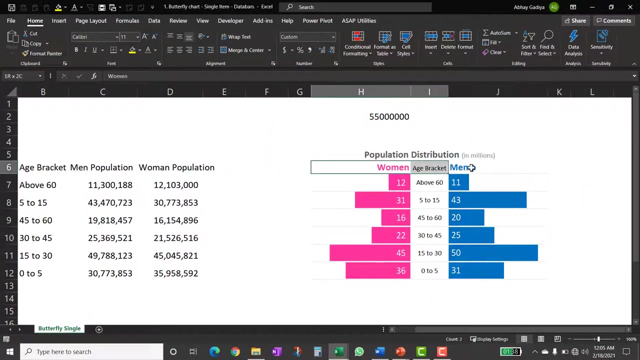 This can have a little different color, So this looks proper to me. So this is done. Now let us quickly add borders to this. So let me quickly select this one, Then I will select this and quickly add the horizontal lines. So this way it looks proper. 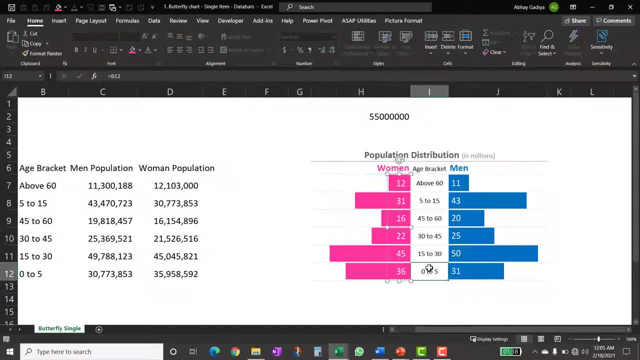 Here also we can quickly add. So this looks proper to me. Now, when you are going to put this chart somewhere else, you can't like just copy this formula again and again. So again we will have to use the trick which we have done for link chart. 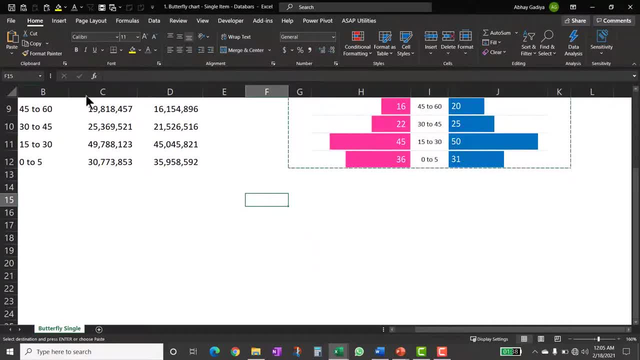 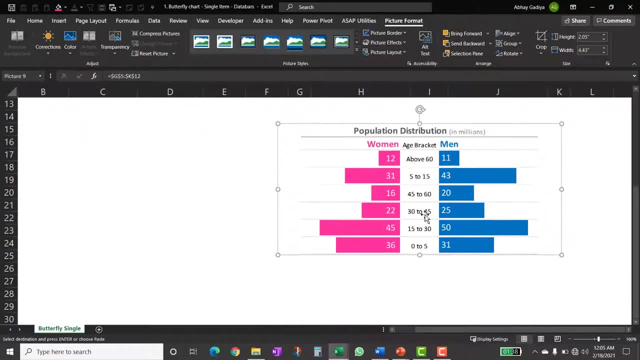 So let us quickly copy it. and then anywhere in this excel sheet I can put link picture. So whenever there is a change here it will automatically gets displayed here as well. So for an example, let us say, if I change a number here, 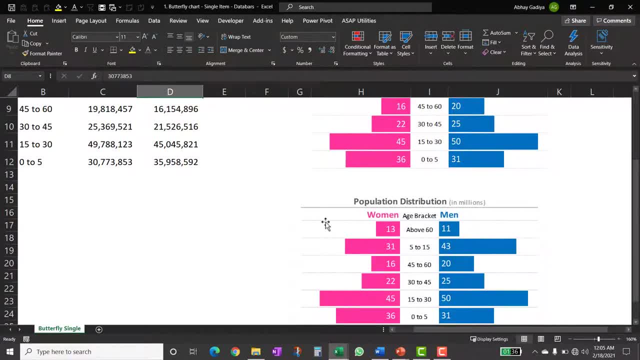 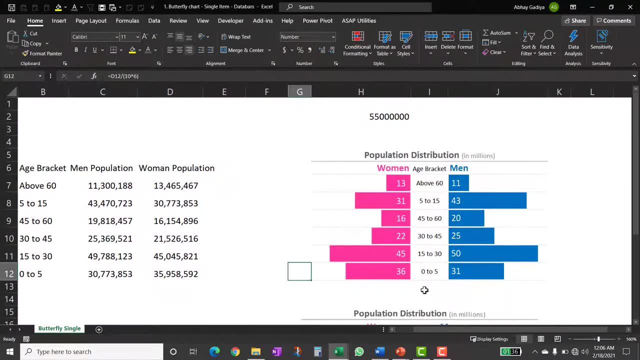 So immediately you men is displayed And here also the numbers will get updated. So this way you can use your link picture and create this butterfly chart in excel using data bars. So that's it like from my side, guys, for this video. In next video we will be seeing second approach of creating this butterfly chart using horizontal. bar charts. So see you guys in next video.